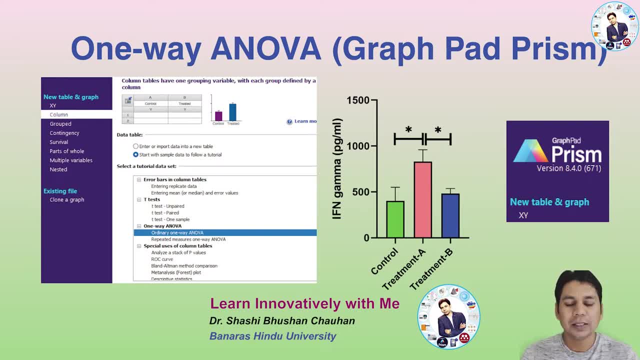 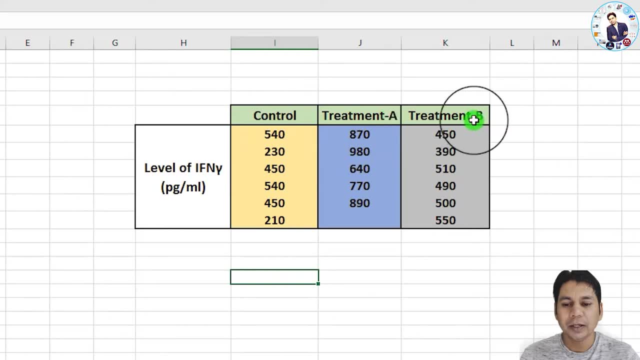 are significantly different or not. So you can see on my laptop screen. Here I am showing a data level of interferon gamma in control treatment A and treatment B group And you can see the data in all three groups. So how you can do one way, ANOVA test using graphpad prism software. 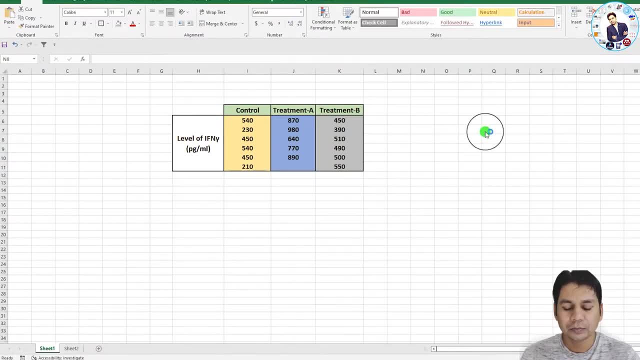 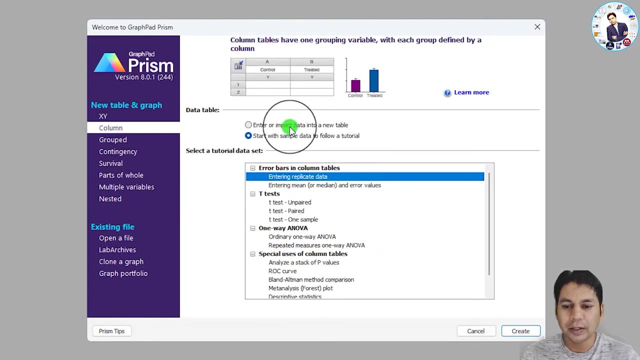 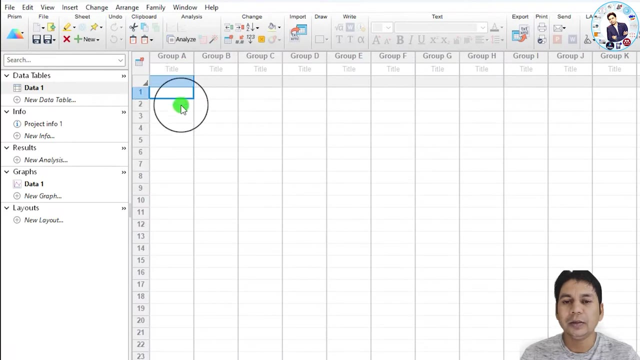 For this, open your graphpad prism software In the graphpad prism software in the column. if you click here on the enter or import data in a new table and click on create, this will open the panel in which you can put your data in the respective group. But 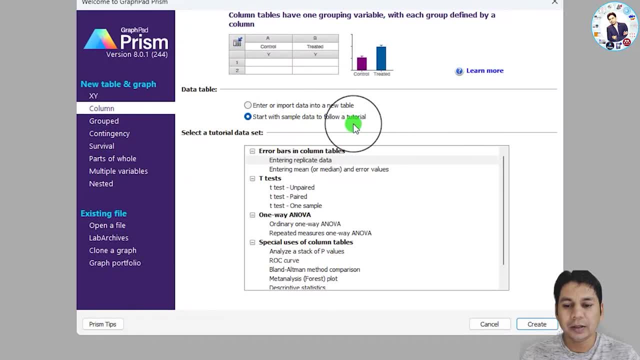 if you click on create, this will open the panel in which you can put your data in the respective group. But if you click here on the start with a sample data to follow it tutorial, and here it is extended, but maybe in your case it is minimized. So to show the option, click here on the plus button. you can see the option. 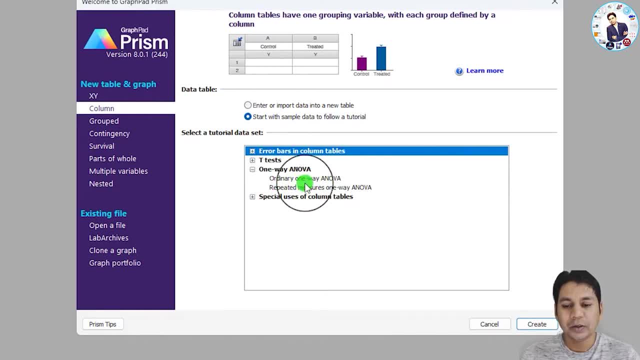 So in one way ANOVA there is two option: ordinary one way ANOVA and repeated measure one way ANOVA. So today I am going to discuss about only ordinary one way ANOVA and I will discuss the repeated measure one way ANOVA later in my tutorial. 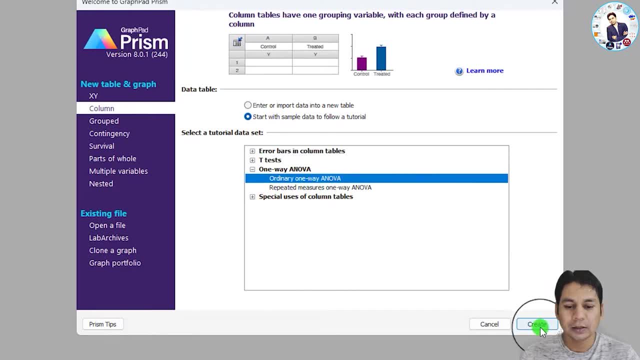 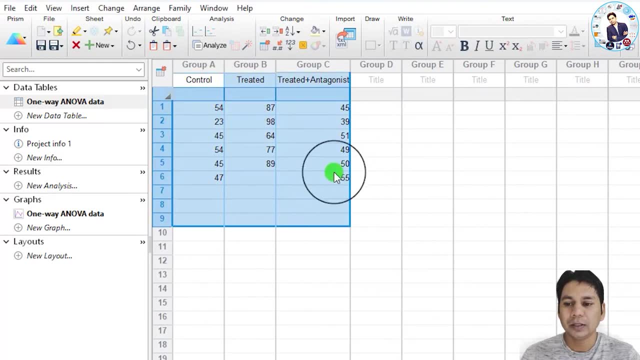 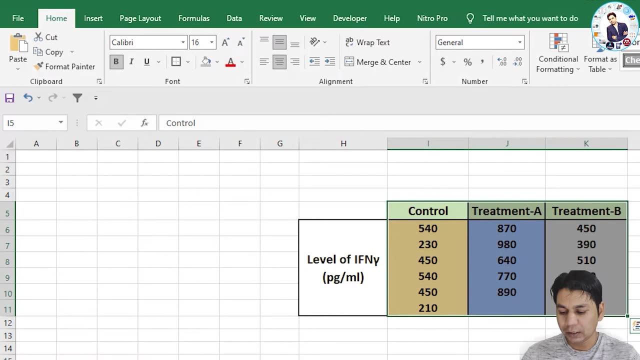 So select this and click on here: create. Here you can see the data already present for tutorial purpose in the graphpad prism software. You can select and delete this data and you can copy your data from the excel sheet and paste in the graphpad prism software. 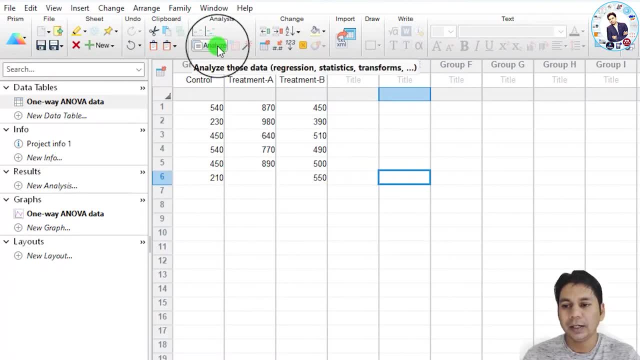 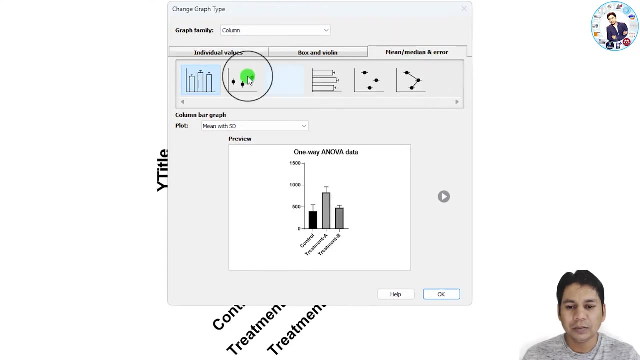 And to analyze the data you can click here on the analyze button and also in the result section, new analysis. But before this you can see the graph of this data if you click here, and here is the option to select the graph type. Here I am selecting the mean, median and error in each. 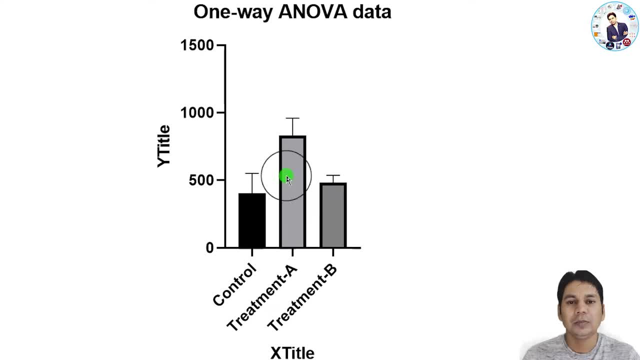 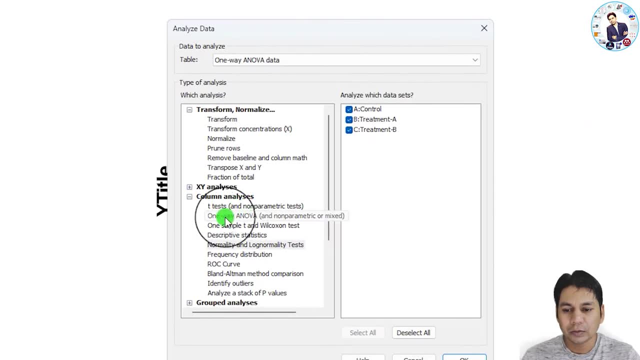 column bar graph You can see the graph of the entered data. and now click here on the analyze button and you can see in the column option one way: ANOVA. click here and at the right side you can see the your sample group. You can select or deselect group. 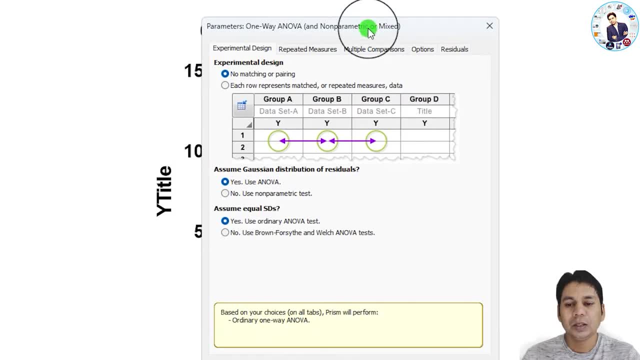 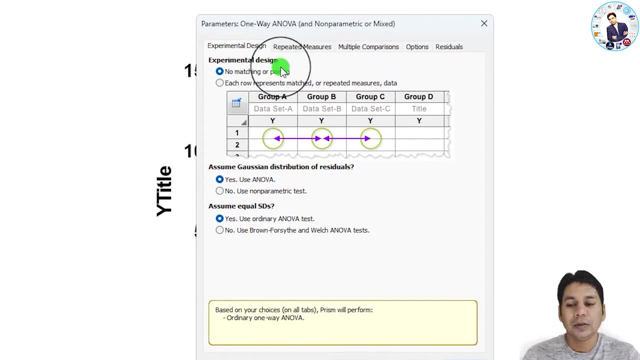 If you select gus, then you go to elements space and click here to select as data. You can also select all equ noon and leaving all ape od data only Click here on the order field. So now you can see theadle requirement as well, and first you can see the experimental design in which you can see there is two experimental design. first, no matching or pairing, so you can see there is no matching in your group data. and if you select the, each row represent matched or repeated measured data. you can see each row representing the paired sample. But in my case there is no matching or paired data, so I am selecting them. 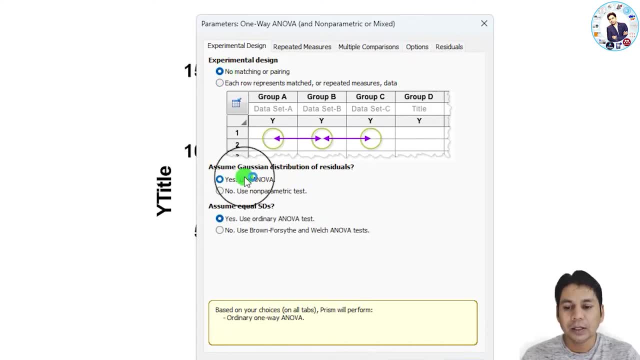 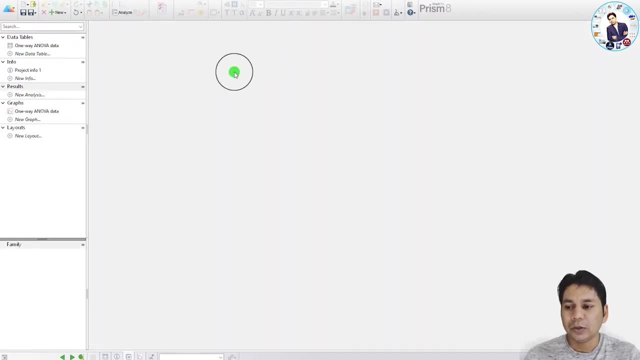 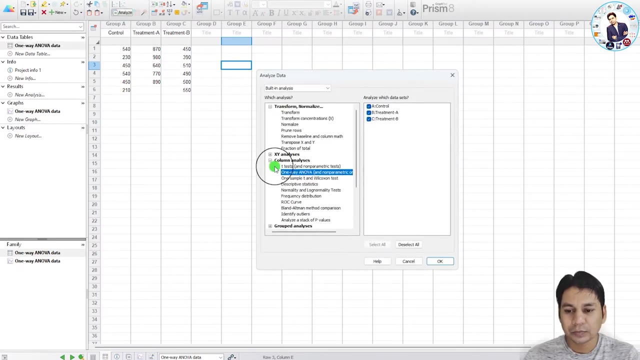 data. so I'm selecting the no matching or pairing and assume the Gaussian distribution of residuals. so for this you can perform a normality test. so I'm going to show you how you can perform the normality test for this. select your data and click here on analyze, and in the quorum analysis. 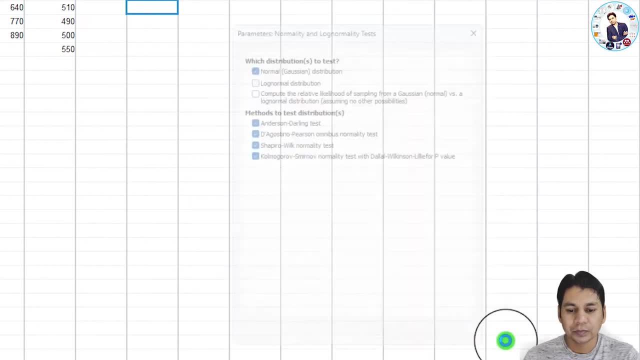 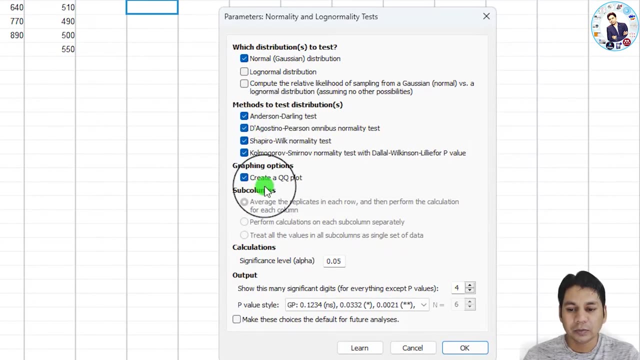 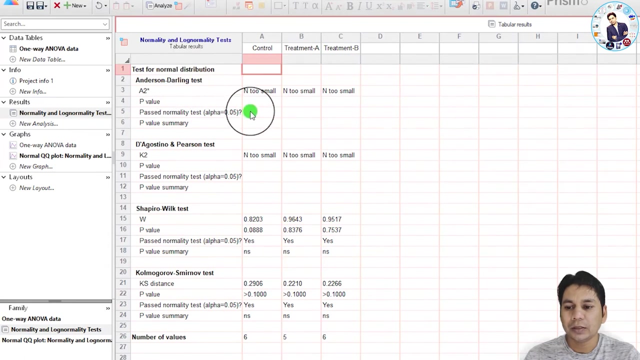 select the normality and log normality test here. click here on ok and here is the option to select the test to analyze the normality. so by default it is selected from all the tests, so I'm not going to change this. click here on the ok and here you can see first two tests showing that there is 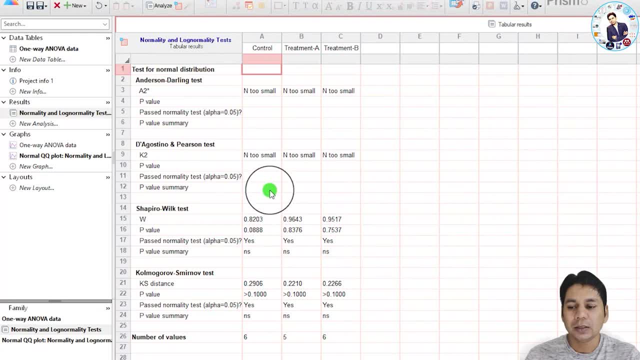 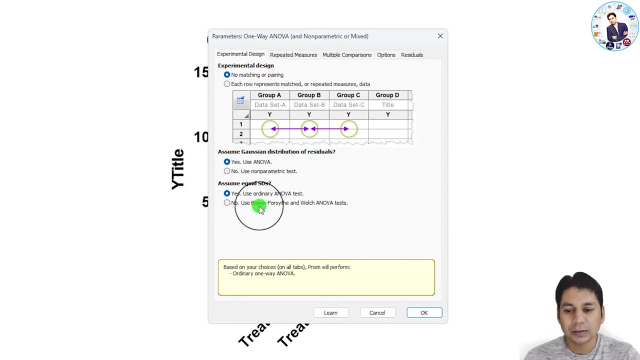 two small sample. that's why they are unable to perform the test. and in the last two tests- here you can see the past normality test: yes, for all three groups. so you can see our data is normally distributed and I am assuming Gaussian distribution of residual. so i'm selecting yes. 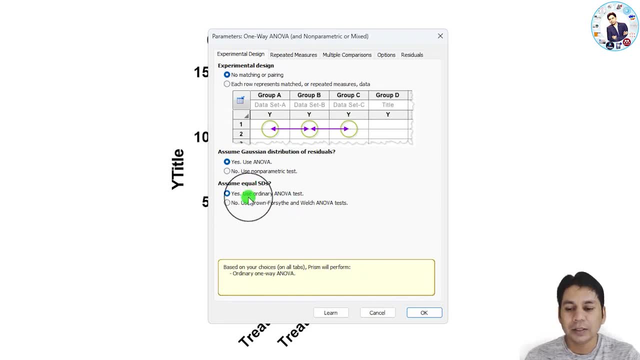 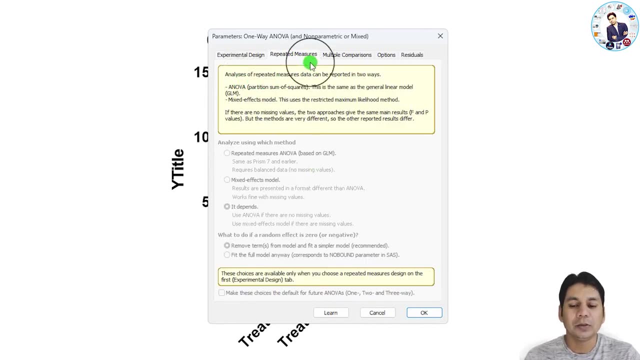 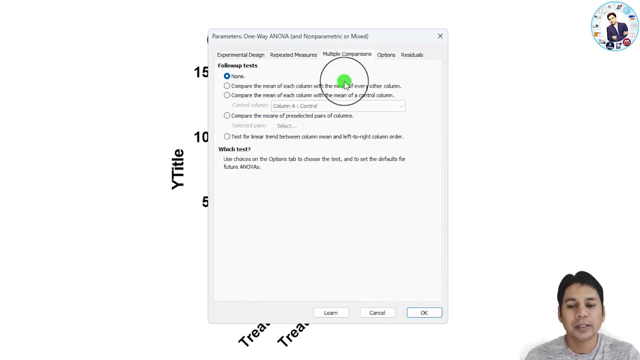 and also for the equal standard deviation. here I am also selecting yes. now if you click repeated measures, as I have not selected for the repeated measure, so here it is not showing anything. so next, click on the multiple comparison. this is for the post hoc test analysis, so by default it is none. but if you click here, 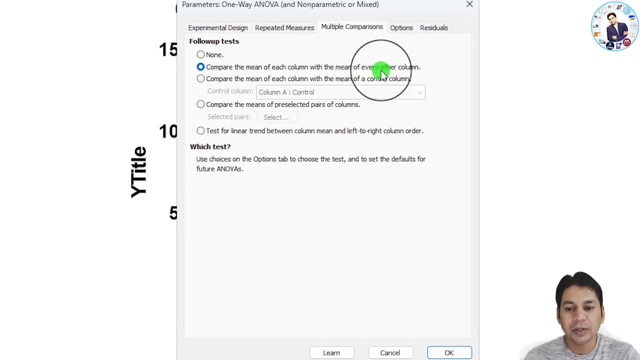 compare the mean of each column with the mean of every other column. if you click here, it also performed the test for the mean of one group with the mean of every other groups. if you select this, but if you select the next one, compare the mean of each column with the mean of control. in this case, it performed the test from: 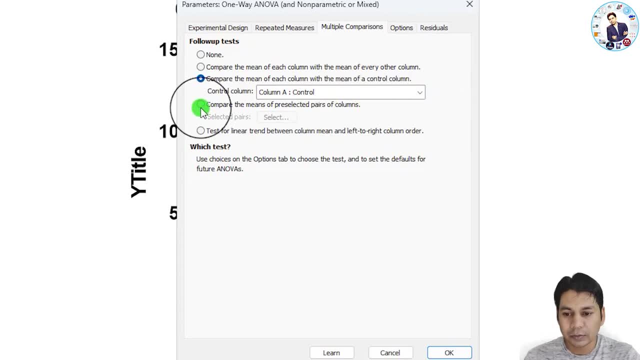 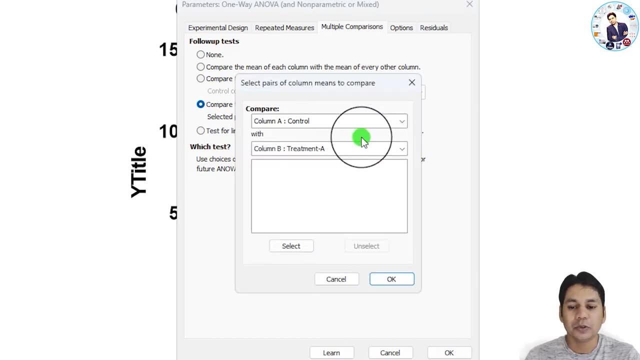 the mean of control group to other groups. and the next one compare the mean of pre-selected pair of columns. so you can select the group in which you want to perform the post hoc test. but I am going to select the. compare the mean of each column with the mean of each column, and the next one compare the mean of. 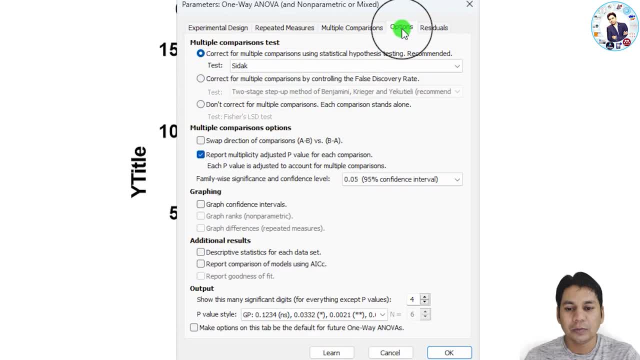 with the mean of every other column. And the next option here is the multiple comparison test. If you select this, you can see there is a Tukey, Bonferrini, Sridhar, Holmes, Sridhar and Newman Quills test for multiple comparison test. 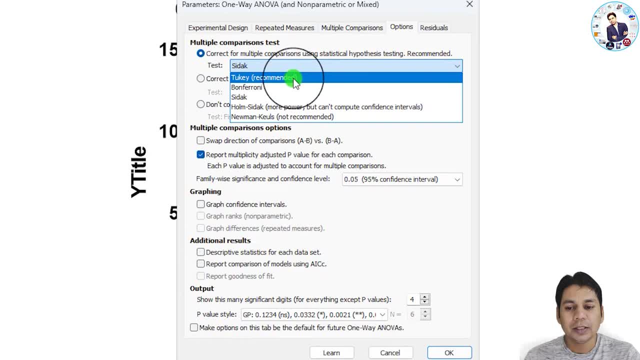 But here you can see the graph pipeline recommending the Tukey test. So I'm selecting the Tukey test for the multiple comparison test, But maybe in your case you can change accordingly And I am leaving with the default value here and in the additional result, if you click. 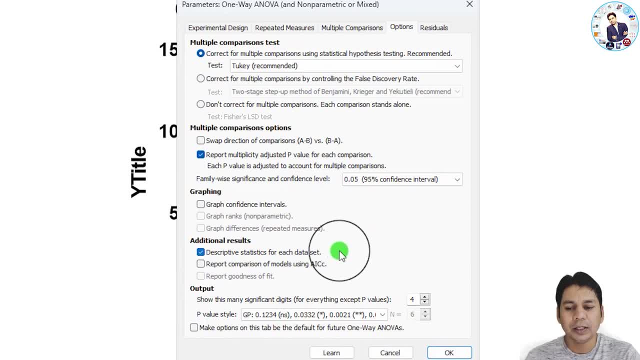 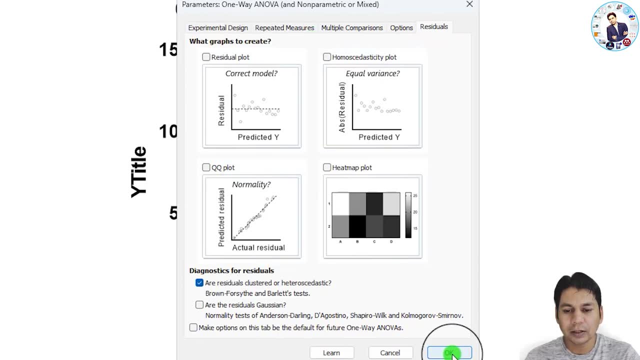 here on the descriptive statics for each data set. the result will be in the descriptive form, also Next residuals. So I am leaving these option and click here on the OK. Here you can see ANOVA result and multiple comparison and here also the descriptive statics. 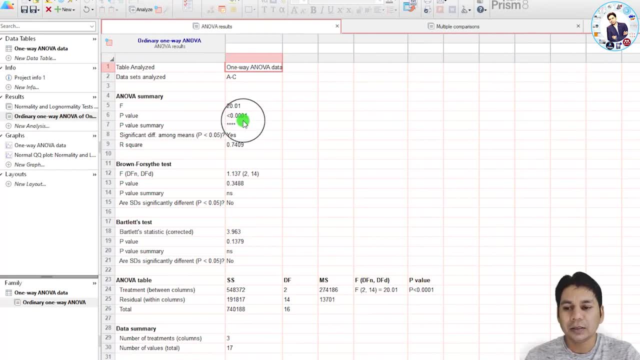 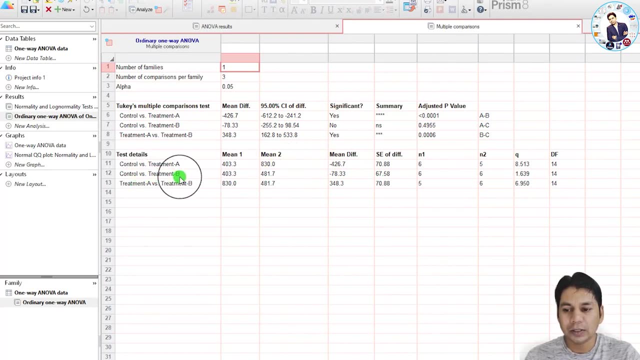 So you can see in the ANOVA result there is a significant difference And if you click here on the multiple comparison, You can see it analyzed: the data: Control vs Treatment A, Control vs Treatment B and also Treatment A vs Treatment B. 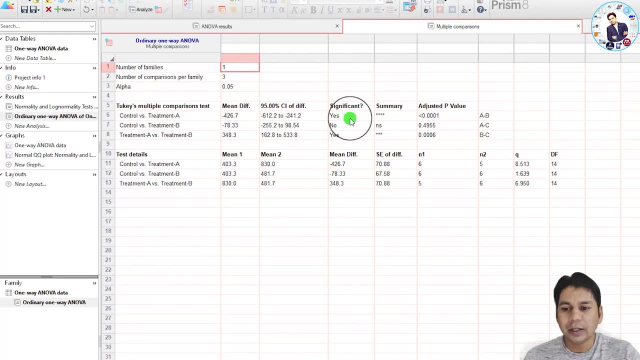 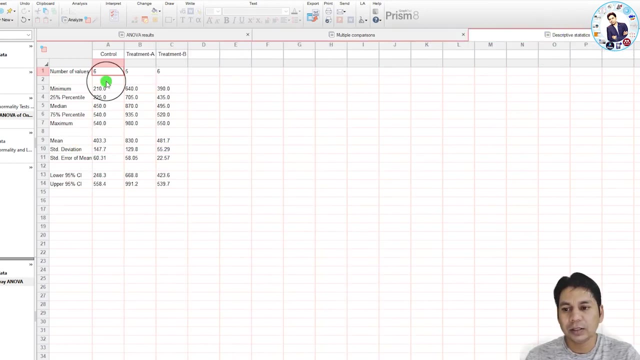 And here you can see the result: Control vs Treatment A have the significant difference and Treatment A vs Treatment B also have the significant difference, But there is no changes between Control and Treatment B. You can see here, And if you click here on the descriptive statics, you can see the descriptive analysis of that. 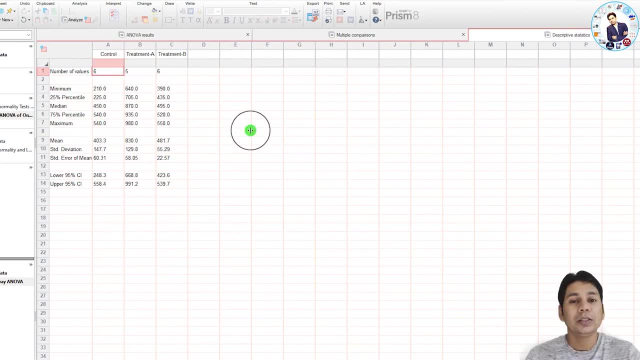 Control treatment A and Treatment B group. so in this way you can perform the one-way ANOVA test in graphpad prism software and i hope this may help you in your research. and if you like the video, please subscribe my channel. thank you.